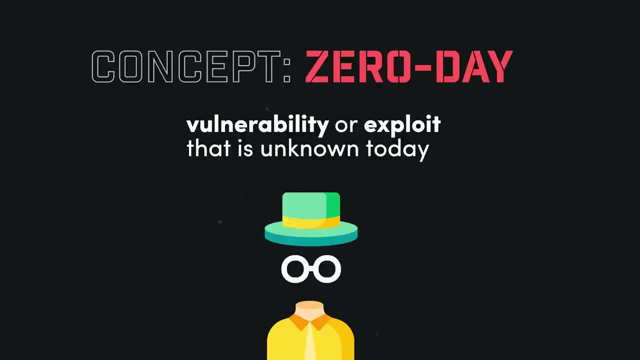 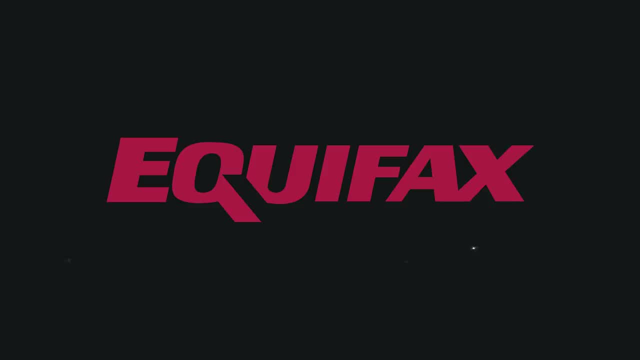 yet been fixed. These are known as zero-day vulnerabilities because, as a developer, you have zero days to get it fixed. When a hacker decides to attack this vulnerability, it's known as a zero-day exploit. Remember that one time, Equifax had exposed the credit. 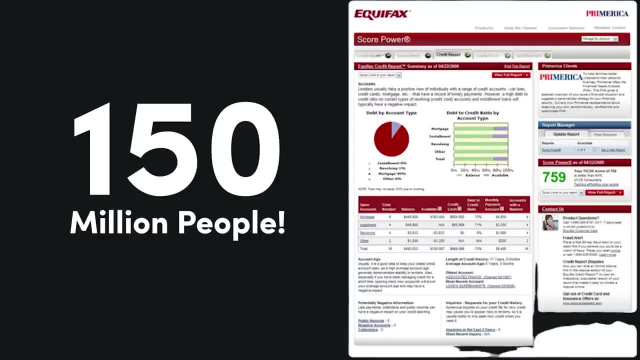 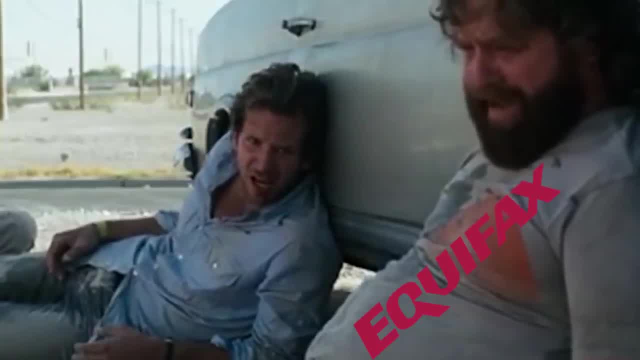 reports of 150 million people. That wasn't the result of a zero-day exploit. It was the result of a known bug in Apache Struts that had already been fixed weeks ago. What, I'm sorry, I fudged up guys. Hackers, apparently from China, had been scanning the web for servers with this vulnerability. They hit the mother load with Equifax and extracted sensitive information over the next 76 days. This breach has cost the company over a billion dollars and could have been prevented by. 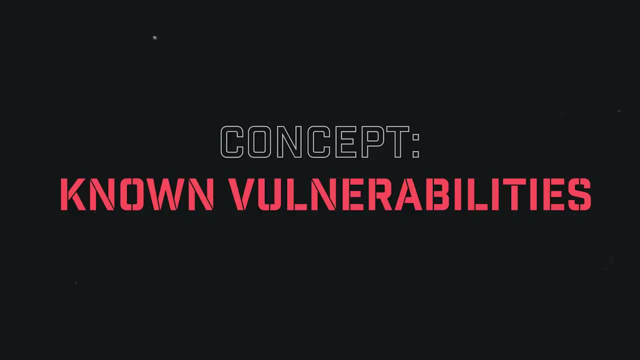 installing a simple security patch. Being hacked by a known vulnerability is not uncommon at all. In fact, you're likely shipping code with a lot of known vulnerabilities right now. If you're a JS developer, go into your project and hit NPM Audit. It will give you a breakdown. 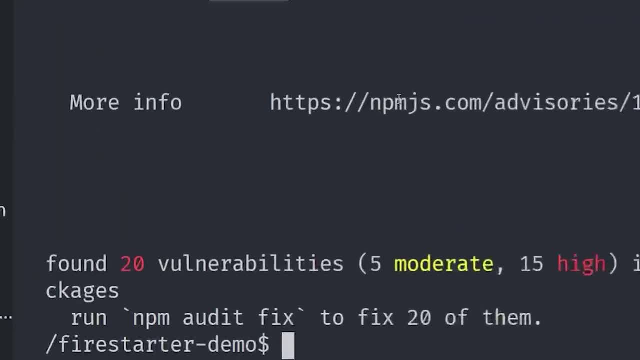 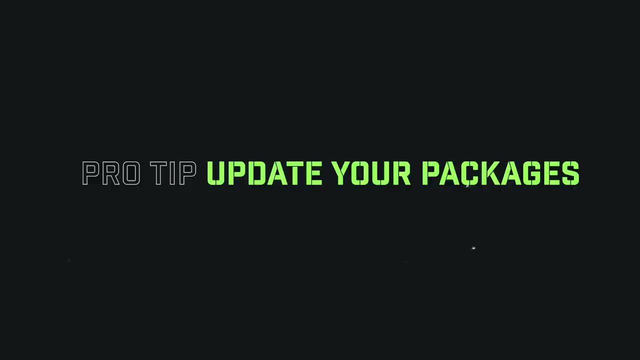 of all the different ways you can be hacked via your open-source dependencies. Now there's no reason to panic If you have hundreds of high-severity alerts. the best way to avoid being hacked is to simply update your packages, But if you truly want to understand the flaws that are compromising these packages, 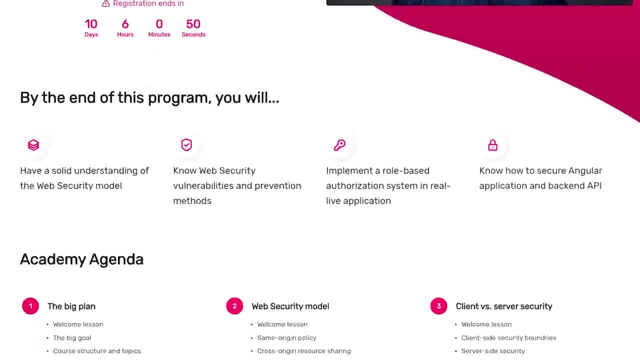 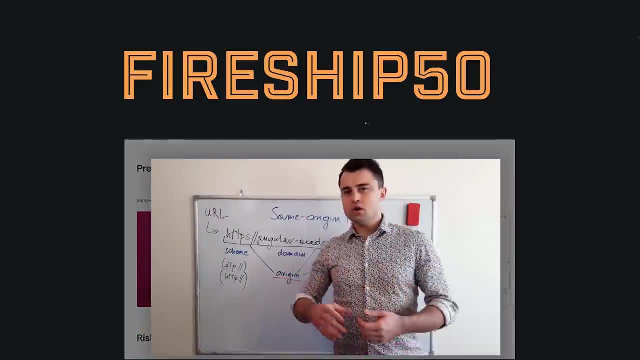 you should enroll in the Enterprise Security Course from Angular Academy. It's a 10-week long program that will teach you how to confidently build secure web applications. You'll find the link in the description and you can use this code to take $50 off the. 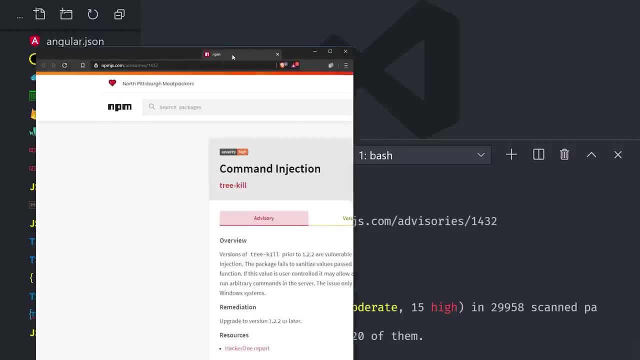 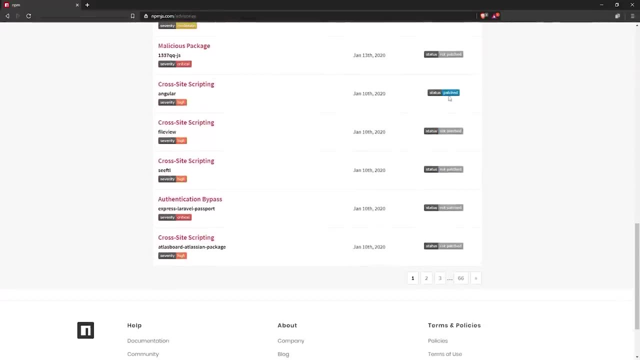 enrollment price. Using components with known vulnerabilities is one of the most common ways that web applications get hacked, But it's also very preventable because, as you can see here, most of the issues have already been patched. And keep in mind, this issue isn't unique to 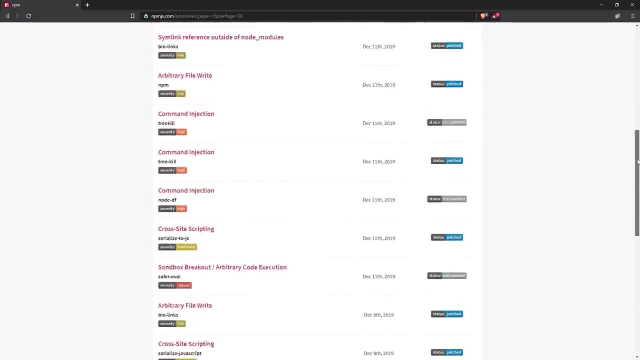 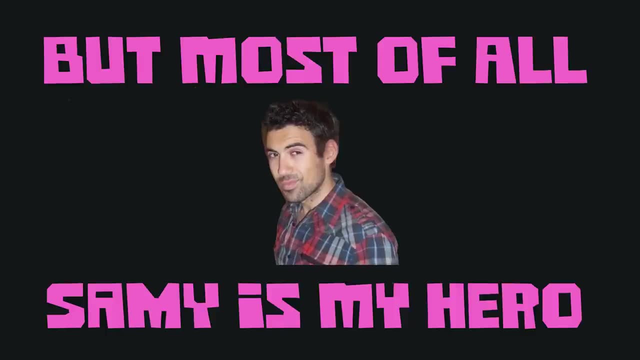 JavaScript or NPM. All package managers that rely on open-source code face similar issues. so trust nobody and keep your packages updated. But most of all, Sammy is my hero. Wait a second. I didn't mean to say that last part. It was somehow injected into this video. 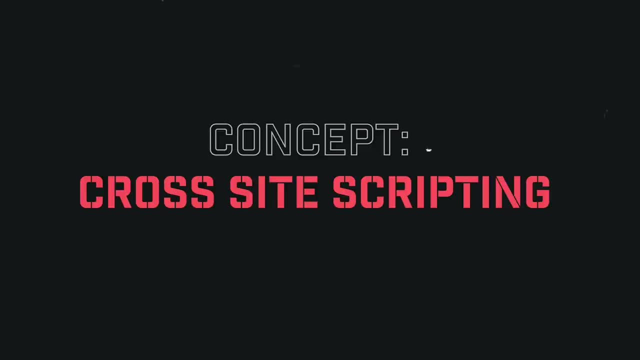 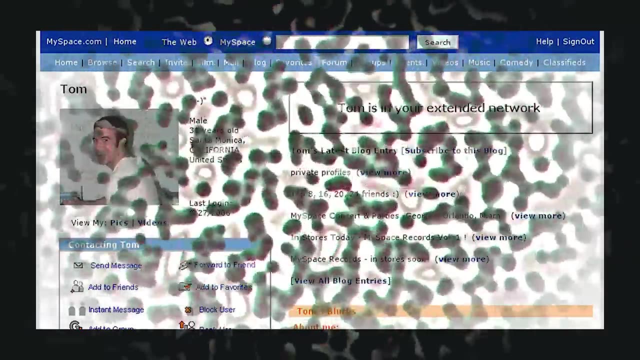 Back in 2005,, a guy named Sammy used an exploit known as cross-site scripting to update a user's MySpace profile with this text. Within a day, it had spread to over a million users. It was mostly harmless, but they did arrest Sammy, convict him of a felony and, worst of all, took away his 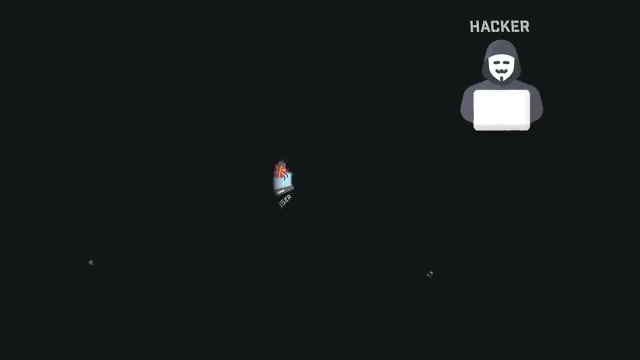 internet for a year. A cross-site scripting exploit occurs when the attacker manages to run some JavaScript code on a different user's browser. There are a few different ways to achieve this, but the most common way is for the attacker to save the script in a web application's database. 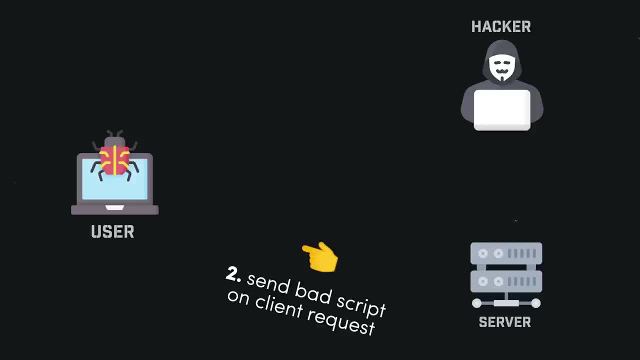 The malicious script will then be accessed by a different user that will execute the JavaScript on the client-side device And at that point, the user will be able to execute the JavaScript on the client-side device And at that point, the user will be able to execute the JavaScript on the client-side. 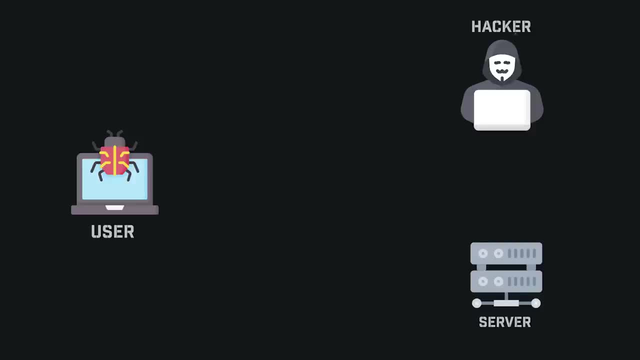 device, And at that point the user will be able to execute the JavaScript on the client-side device, And at that point the JavaScript code can submit forms. click on buttons on behalf of the logged-in user. So how do you avoid cross-site scripting attacks as a developer? Well, the attacker first needs. 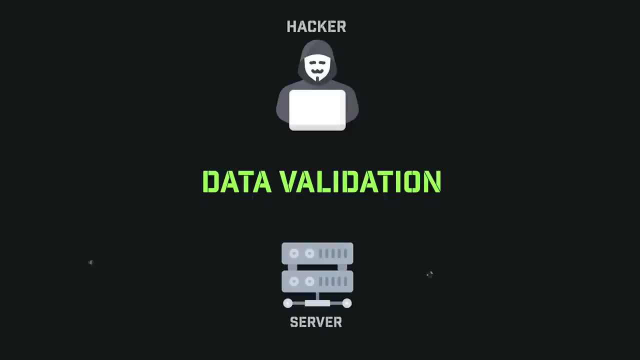 to save some malicious code on your server. So step one is to do some server-side validation of incoming data. If it's surrounded by script tags, you might not want to save it. But let's imagine you fail to sanitize the incoming data. The attacker still needs a way to run that script. 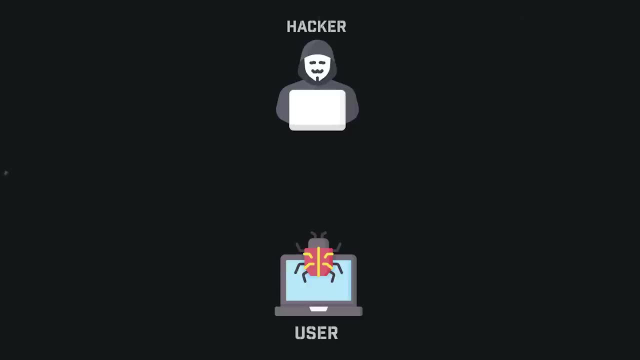 on the client-side device. So the attacker is counting on you to render out the raw HTML of the script. Fortunately, the attacker still needs a way to run that script on the client-side device. So the attacker is counting on you to render out the raw HTML of the script. Fortunately, 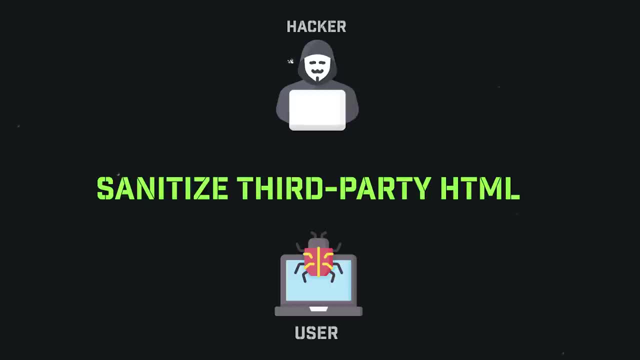 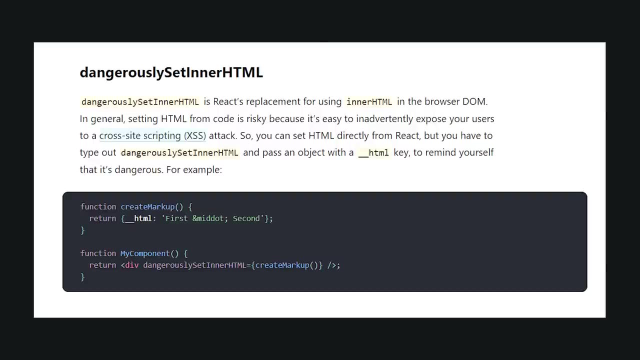 the attacker still needs a way to run that script on the client-side device. Fortunately, modern front-end frameworks make it really difficult to shoot yourself in the foot. In React, for example, if you want to write unsafe code, you have to use this dangerously set innerHTML prop just to do so. 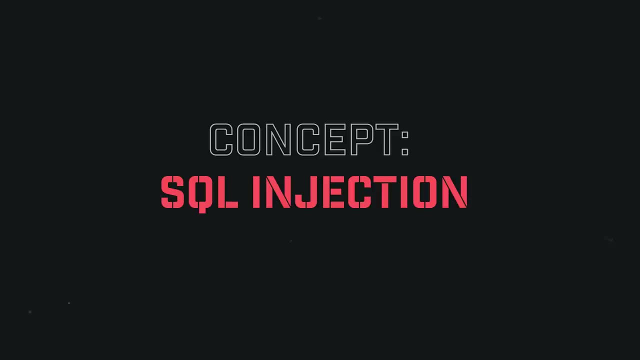 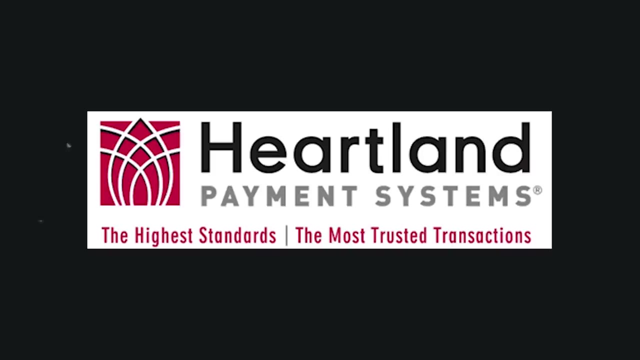 So with cross-site scripting, we have malicious code running on the browser, but it's also possible to run bad code directly on a database. Let's go back to 2008 and look at a company named Heartland Payment Systems, a company with the highest standards and the most trusted transactions. 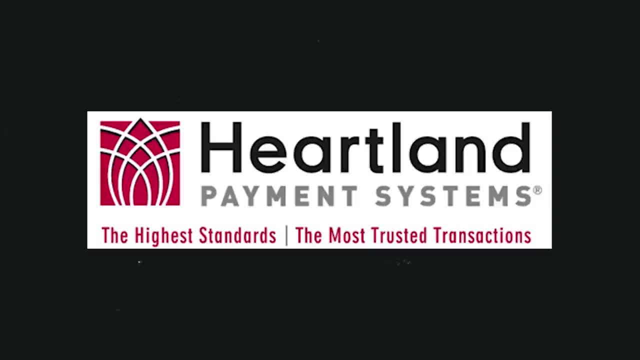 and also a company that was the target of one of the most elaborate and interesting hacks of all time. Let's go back to 2008 and look at a company named Heartland Payment Systems, a company with the highest standards and the most trusted transactions. 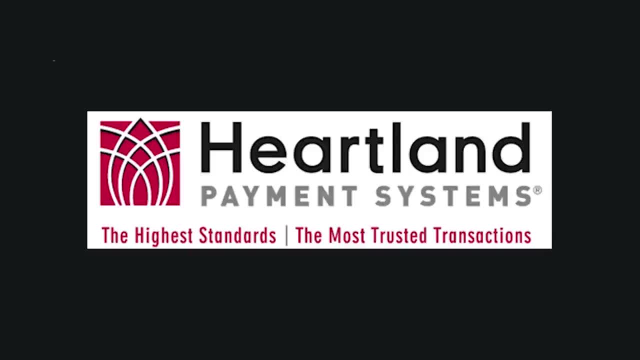 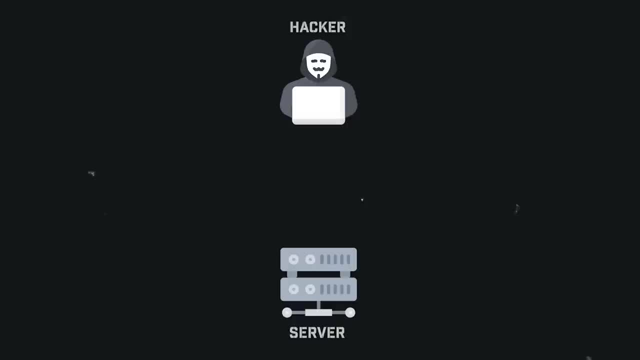 and also a company that was the target of one of the most elaborate and interesting transactions. The attackers first gained access to the company's databases by using a technique known as SQL injection. Instead of sending the expected data to the database, they sent raw SQL statements. 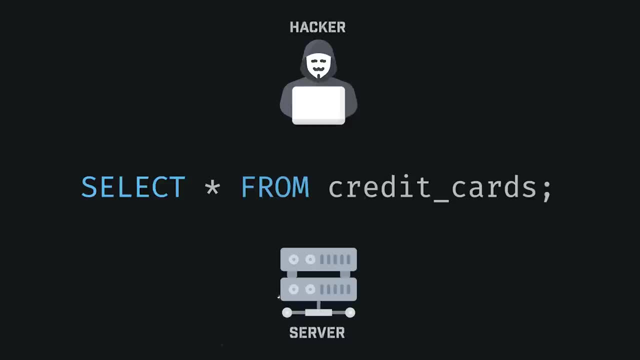 And because the data was not validated, the database would run this code as if it came from the developers. Now, this particular database contained the information that you would find on the back of a magnetic strip on a credit card, And they used this stolen data to create. 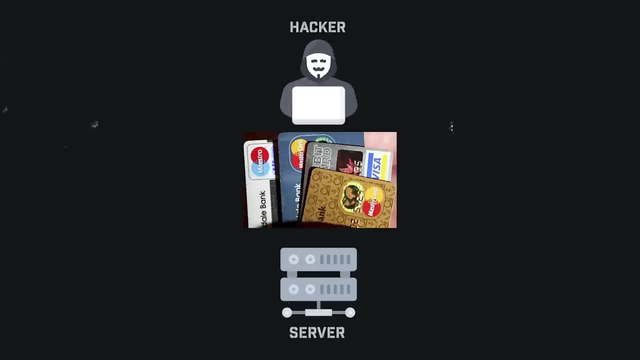 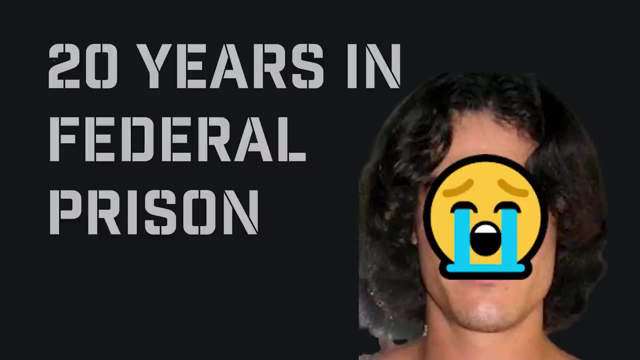 counterfeit credit cards that actually worked. It's estimated that over 100 million cards were compromised and the main hacker, Albert Gonzales, was sentenced to 20 years in prison. Injection attacks similar to this affect many different types of databases. If you use an ORM or object relational mapping tool for your database, 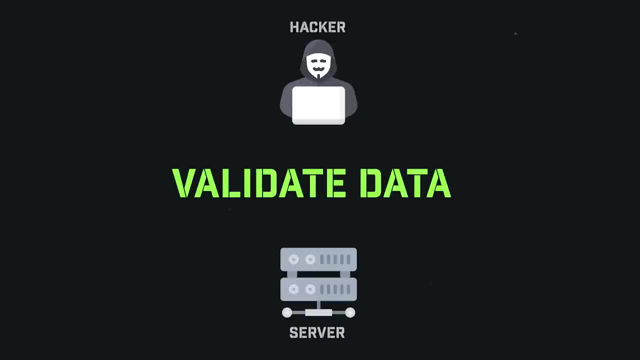 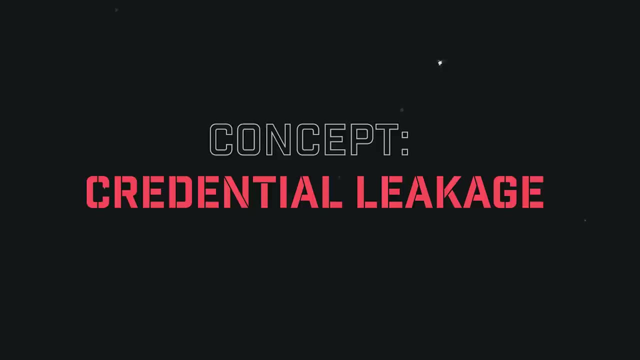 you should be safe from attacks like this, But of course it's always a good idea to validate your input before it's sent to your database. Another very easy way to create a big problem as a developer is to expose or leak a sensitive API key. You can think of a private API key as a username. 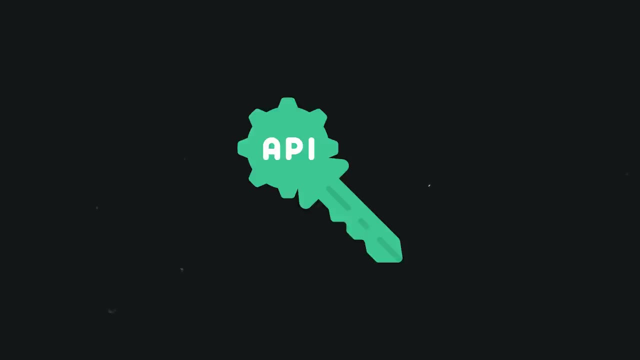 and password all bundled up into a single string, and it allows your servers to securely communicate with paid services like AWS, Google Cloud and so on. A few years ago, I accidentally leaked my AWS API key and it was almost really bad. I was using the Node SDK for a service that required. the API key. I hardcoded the API key directly in the source code instead of setting it as an environment variable. I then proceeded to push the source code to a public GitHub repo. A few weeks went by, and then, all of a sudden, I get a notification from AWS that I've maxed out. 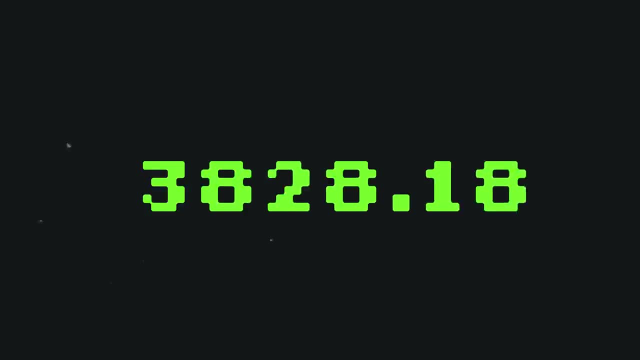 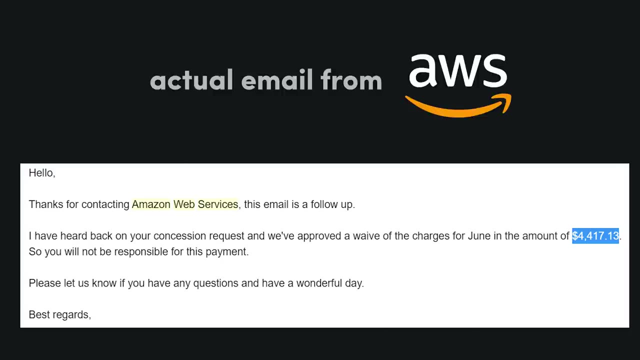 my budget. When I log in, I get a notification from AWS that I've maxed out my budget. When I logged into my AWS account, I had racked up charges around $5,000 for EC2 instances running all over the world. Luckily, Amazon was nice enough to refund those charges, but it definitely 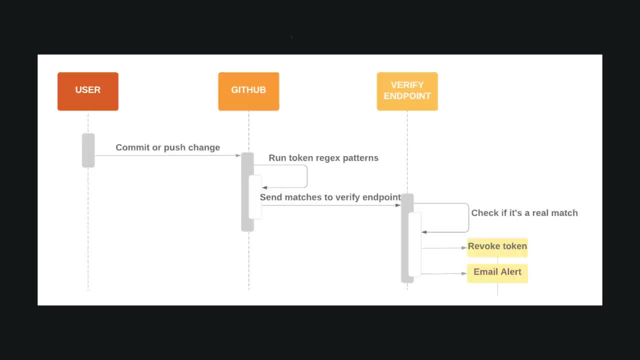 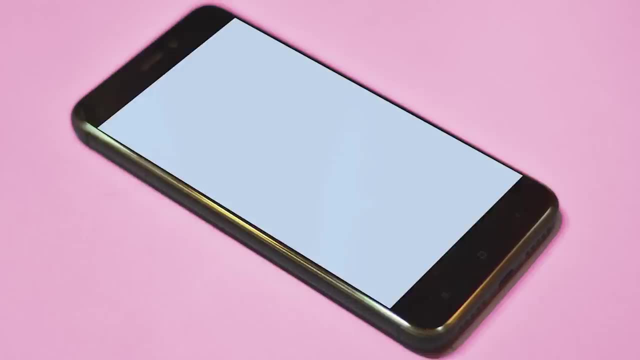 made me feel like an idiot. Nowadays, automatic scanners can often detect if you have an exposed API key and email you a notification. But GitHub isn't the only place that you might leak an API key. When you include a private key in a client-side web or mobile app, a hacker might be. 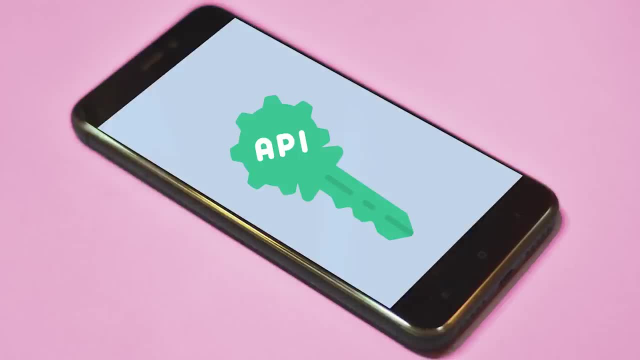 able to find it directly in your source code. Now, if you do end up with an exposed API key, you can fix the problem by simply logging into your AWS account and then logging into your AWS account. You can also do this by simply rolling it to a new value and, of course, removing it from any 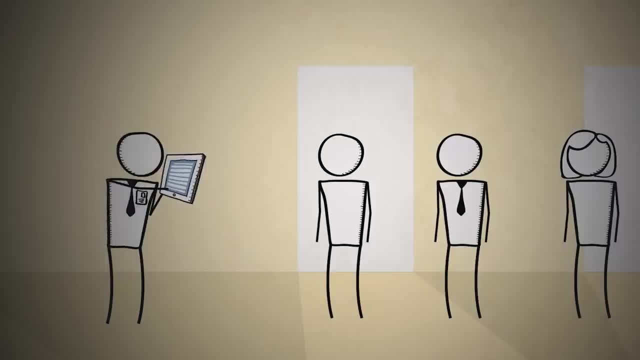 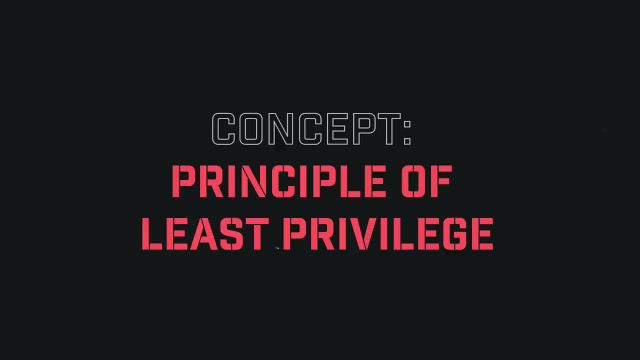 public repos or source code. Many good APIs will help you minimize the damage by allowing you to assign privileges to a specific API key. This allows you to follow the principle of least privilege and only give API keys access to the resources that they actually need. That will 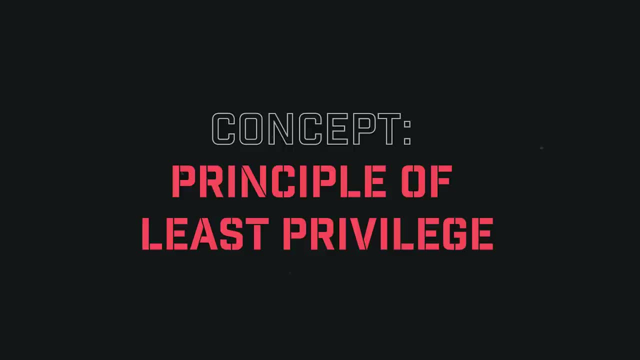 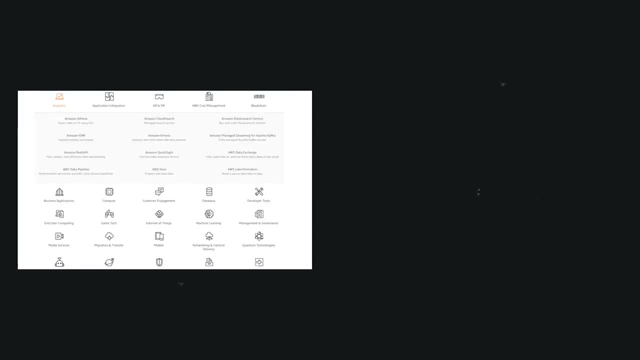 mitigate the amount of damage that can be done if that key does end up being leaked. If we look at a major cloud provider like AWS, we'll see that they offer hundreds of different services And they might be used by a company with thousands of employees working on different. 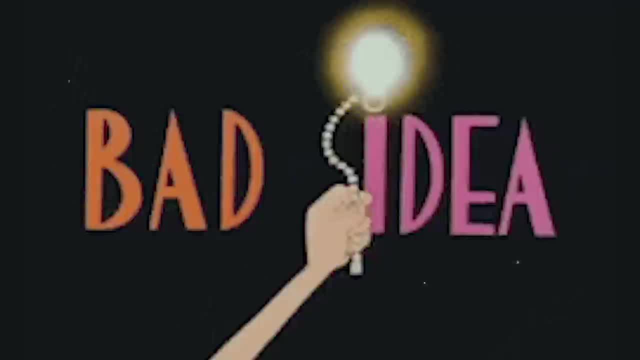 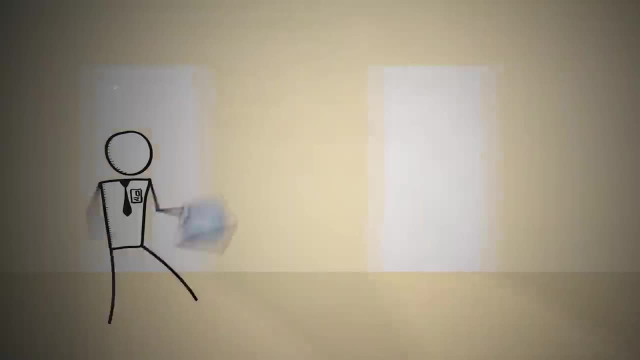 projects. Sharing a single API key that has access to everything would be a very bad idea. Instead, the major cloud providers have a system called IM, which allows you to create groups or roles for your organization. Once you've created a role, you can then attach a policy to that role. 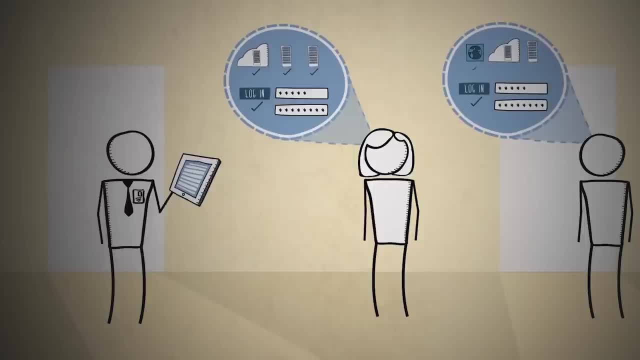 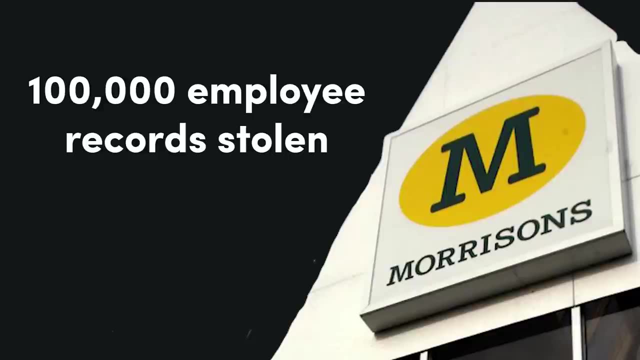 to give it access to a service that it needs Implementing fine-grained access. control over your data is more important than ever. In 2016,, an employee of Morrison Supermarkets in the UK stole the private data of over 100,000 employees. This rogue employee did it by simply. 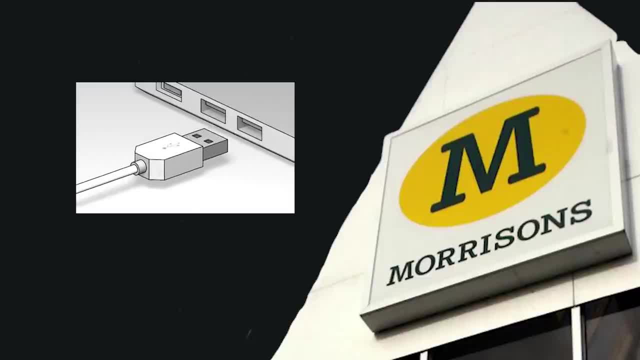 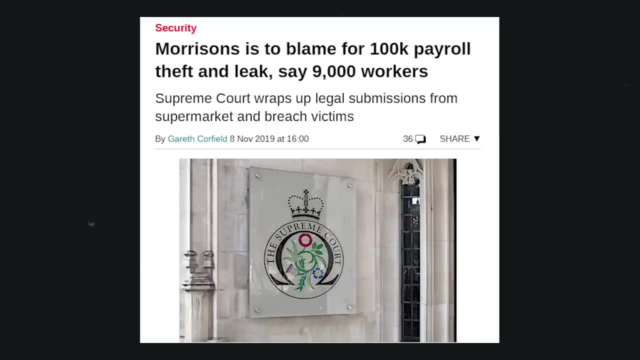 copying the data onto a USB stick. Now, this is obviously unethical and illegal on the employee's part, but the company itself is facing a huge lawsuit and the penalties for data breaches are becoming larger with laws like GDPR and the EU. So the bottom line here is to always follow. 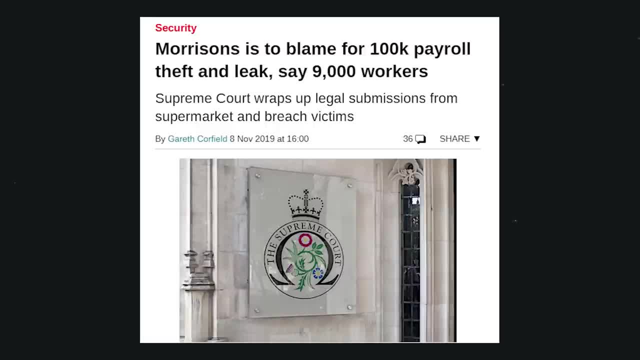 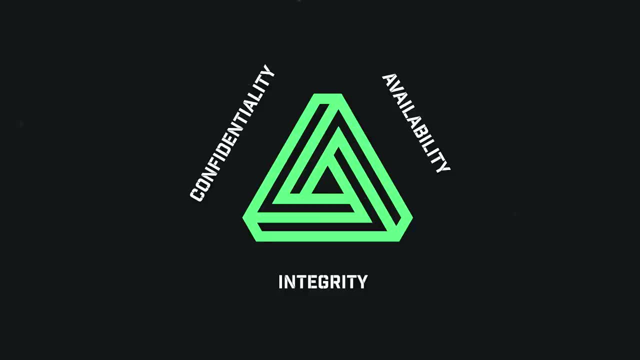 the principle of least privilege when it comes to accessing your customer or employee data. And speaking of data, you might come across something called the CIA Triad. It's a model for data security that stands for confidentiality, integrity and availability, Generally speaking. 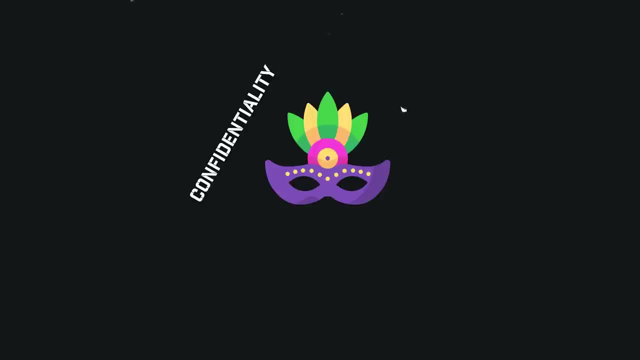 you make data confidential by implementing user authentication, so only authorized users can access the data. Integrity means the data can't be accidentally modified or deleted without the user's authorization. But I think the most interesting question is: how do you make your data highly available? In 2018, GitHub survived the biggest DDoS attack or distributed denial of. 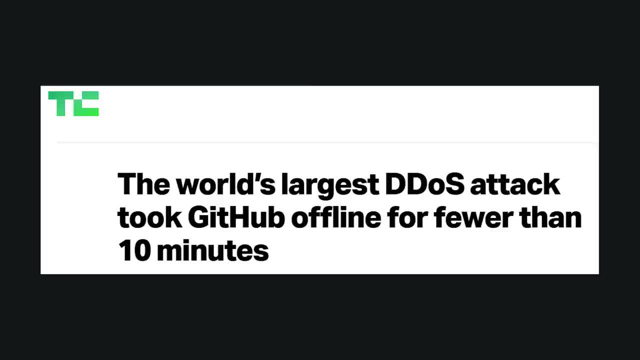 service attack in history. It took GitHub down for less than 10 minutes, but that's still a pretty big deal considering how many people around the world depend on GitHub at any given moment. A DDoS attack was exposed to the public as a result of the DDoS attack. However, the DDoS attack was not. 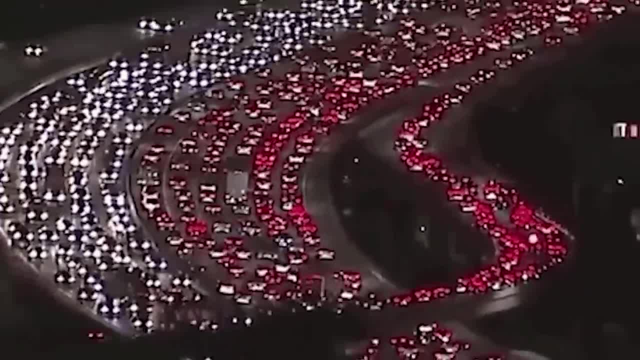 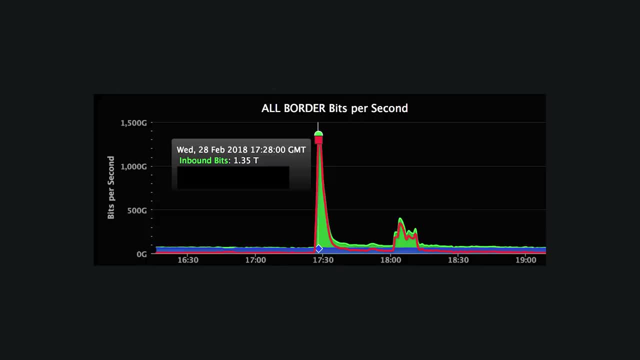 a big deal. The DDoS attack was caused by flooding a service with so much traffic that it just fails to scale and completely stops working. You can see in this chart how the inbound traffic suddenly spiked, but the servers treated these as legitimate requests and responded with a normal response. GitHub is big enough to handle attacks like this, but smaller sites might not be so lucky. In some cases, DDoS attacks have been used to shut down a service and then request a ransom from the owner. So how do you protect yourself? Well, the simple answer is to be ready to scale. 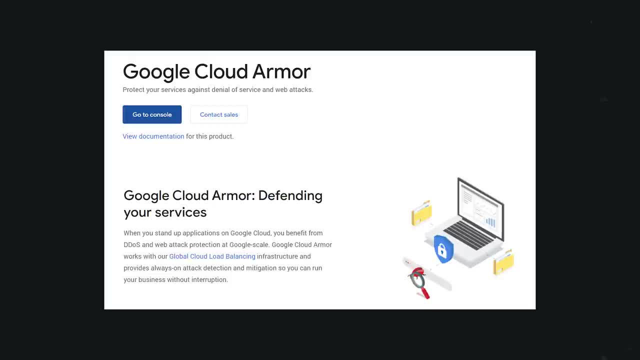 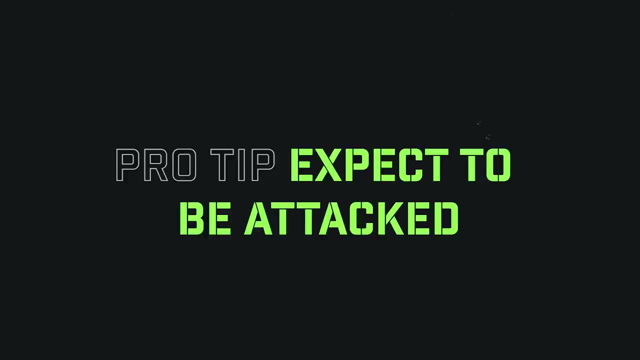 and that likely means using a big cloud provider. A service like Google Cloud Cloud Armor has the bandwidth to handle attacks like this, and it can also prevent many other attacks that we talked about earlier in the video, But at the end of the day, nobody's application is 100% safe. There are likely hackers out there. 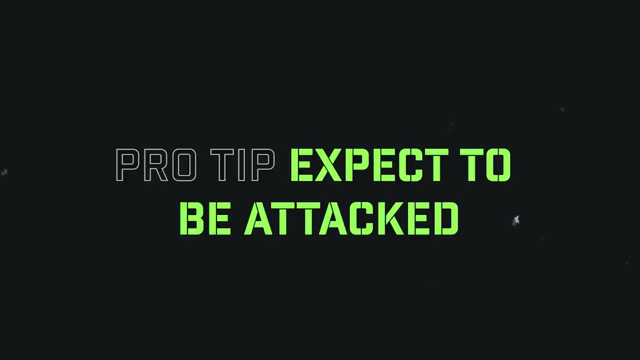 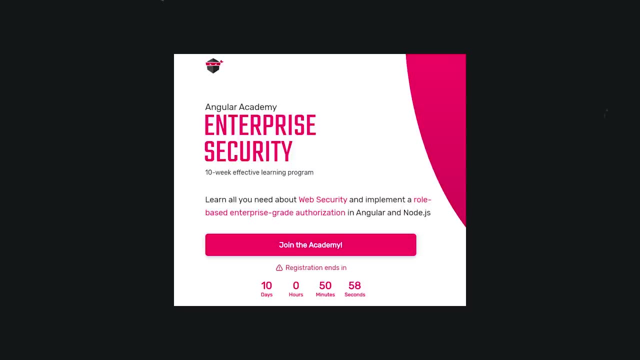 right now using zero-day exploits that we don't know about yet, And it's only a matter of time before the next major data breach is in the headlines. If this video helped you, please like and subscribe, and make sure to check out the Enterprise Security course. 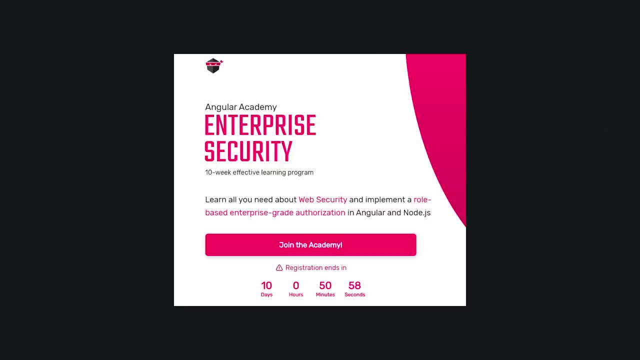 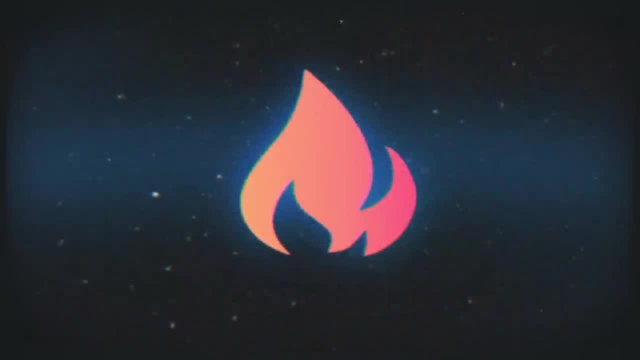 if you really want to master these concepts. Thanks for watching and I will talk to you soon. Bye for now.